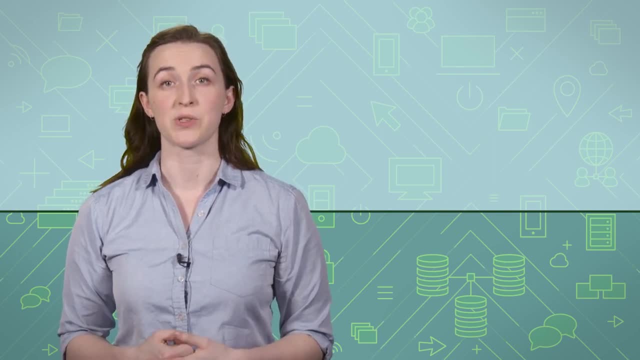 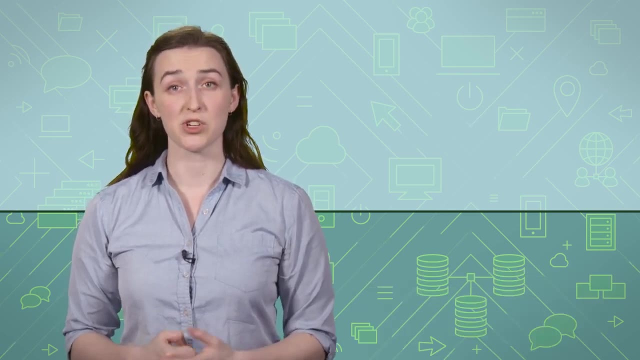 large. If you were to load all of these images at once, it could put a strain on your system's resources. Two: to act as a protection proxy in order to control access to the real subject class. A protection proxy can be used in a learning management system that checks the. 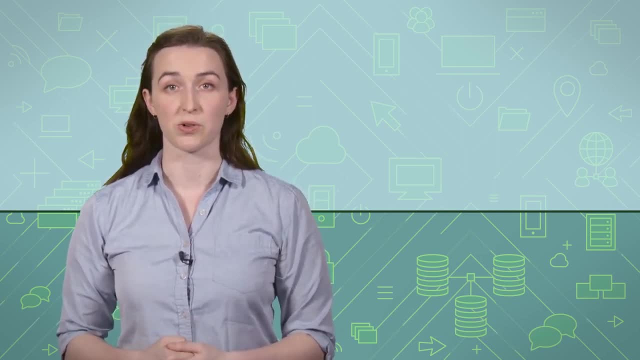 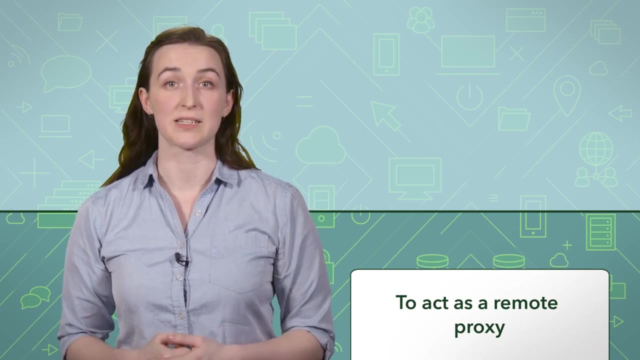 credentials of a user, so that different users, like students and instructors, can access only the appropriate functions permitted by their role. And three, to act as a remote proxy, where the proxy class is local and the real subject class exists remotely. Think. 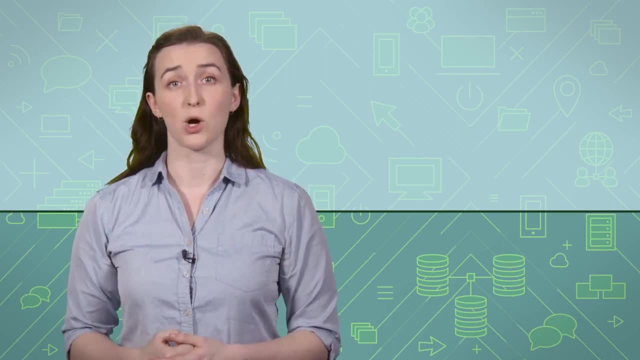 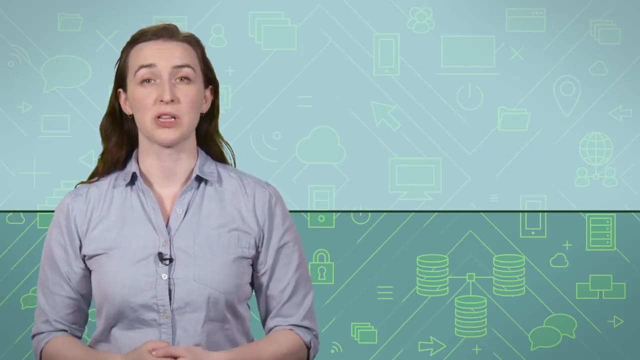 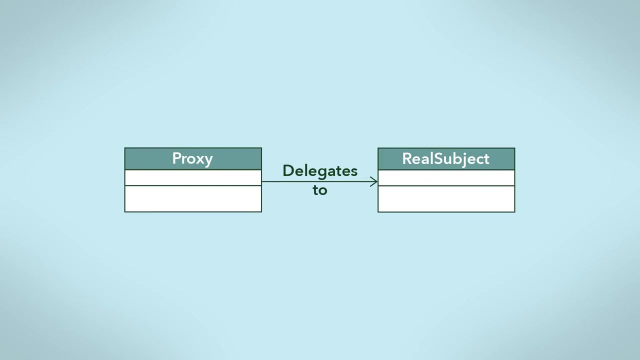 of this like working on a Google document, where your web browser has all the objects it needs locally which also exist on a Google server somewhere else. Let's take a look at the general classes and structure of the proxy design pattern. The proxy class wraps and may delegate or redirect, calls upon it to the real subject class. 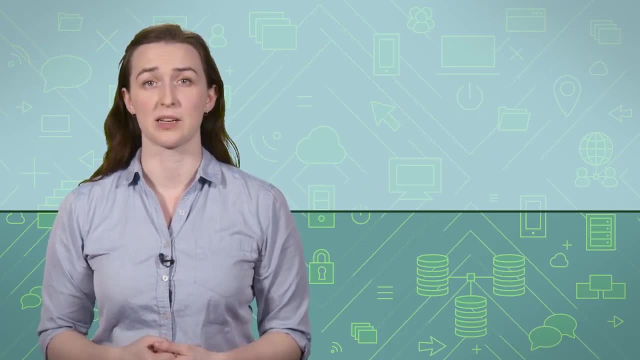 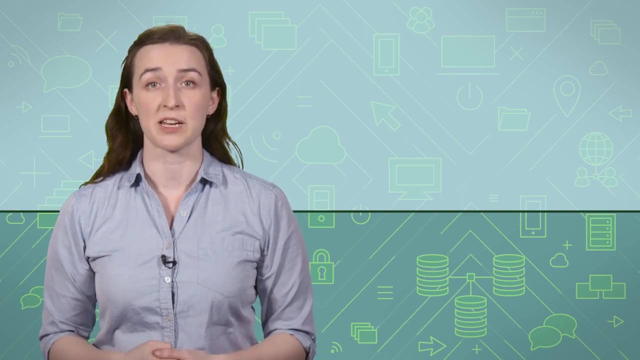 However, not all calls get changed. The proxy class is supposed to act as a lighter version of the real subject class and can do some of its lighter responsibilities. The proxy class will only redirect more substantive requests to the real subject class, But what calls need to be supported in the proxy class? 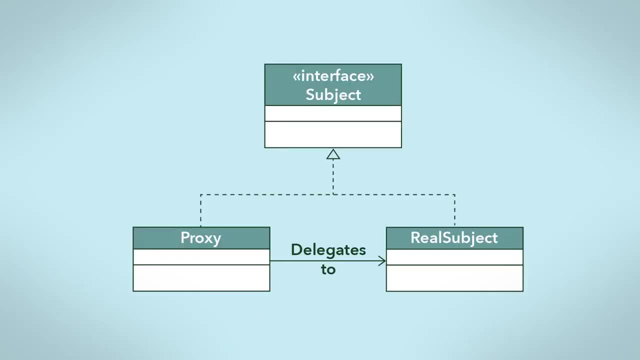 Since the proxy class is meant to stand in for the real subject class, it must offer the same methods. You can ensure that by having both these classes implement a common subject interface which also allows for polymorphism, Since the proxy and real subject classes are. 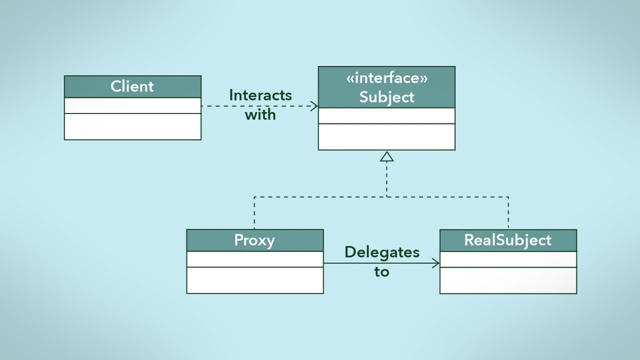 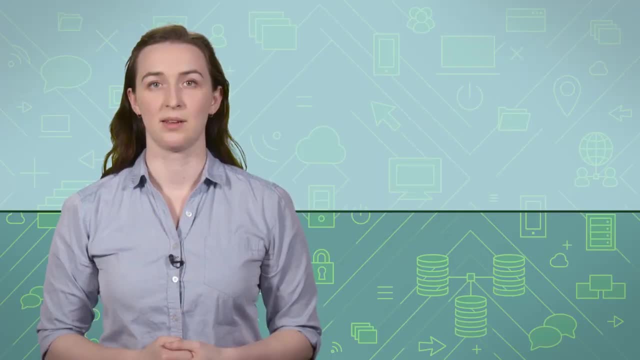 both subtypes of subject. the proxy class is meant to stand in for the real subject class. Since it is meant to be a subject, a client class can interact with the proxy, which will have the same expected interface as the real subject. Let's take a look at a practical application of the proxy pattern. 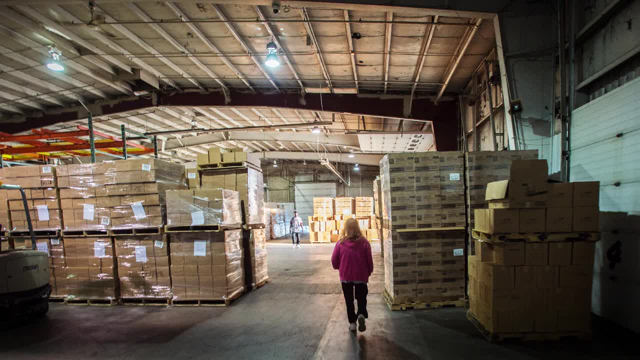 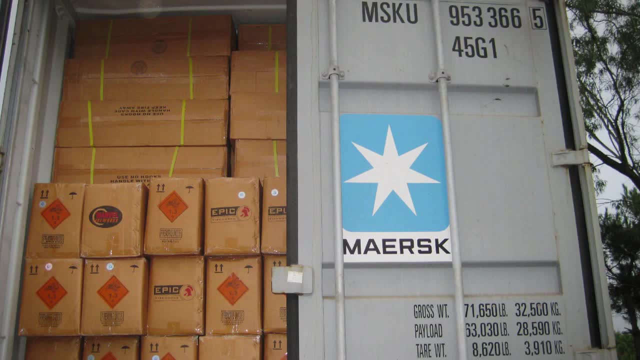 Suppose that you run an online retail store with global distribution and warehousing. How would you know which warehouse to route orders to to fulfill customer orders? You may run into an issue where you route orders to a warehouse that doesn't have stock for an item in a customer order. You need some way to determine which warehouse. 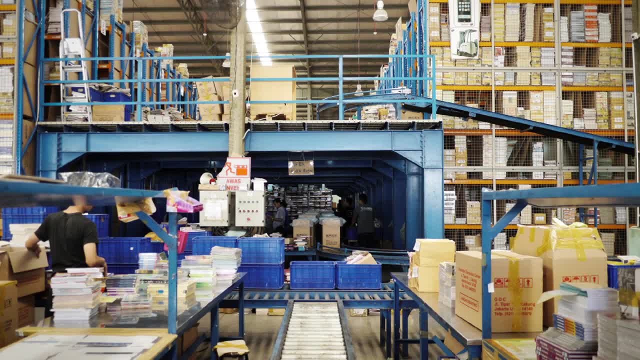 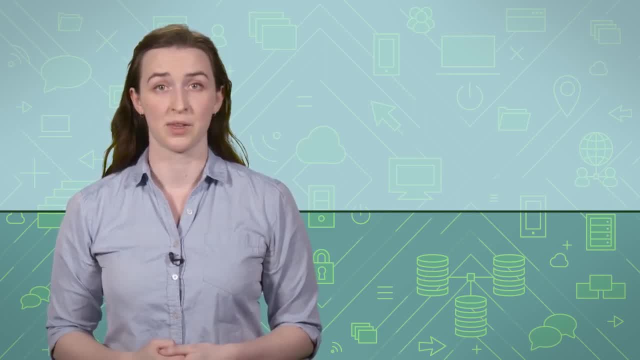 to send the orders to. To do this, you must have an online retail store, which would not to. A system that routes the orders for fulfillment to an appropriate warehouse will prevent your warehouses from receiving orders they cannot fill. So how would you implement this system? You can use the proxy design pattern to have a 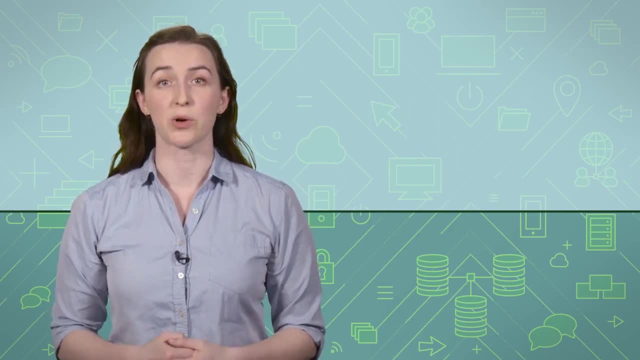 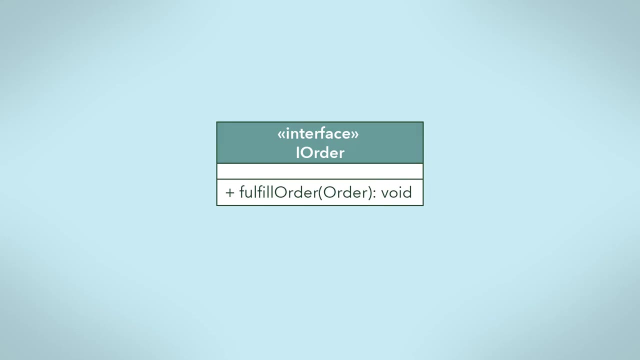 proxy protect your real subject- the warehouses- from receiving orders if the warehouses don't have enough stock to fulfill an order. The IOrder interface defines how you would fulfill the orders. The proxy class and the real subject class will implement the interface differently. 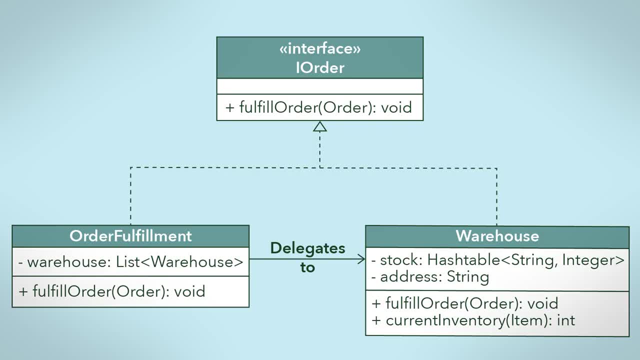 This interface declares how to interact with your order fulfillment system. The Order Fulfillment class acts as the proxy for all your warehouses. It has a list of warehouses that it can delegate parts of customer orders to, depending on whether or not a warehouse is capable of fulfilling. 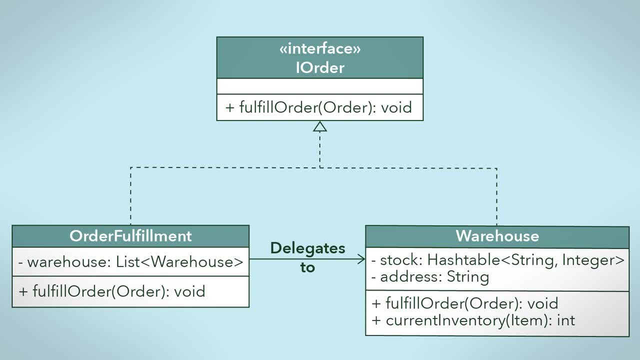 a part of the order. The Warehouse class is your real subject class and will be responsible for actually processing and fulfilling parts of customer orders. The Warehouse class will report its inventory to the proxy that asks for it, As shown in the general design overview for the proxy design pattern, the proxy design. 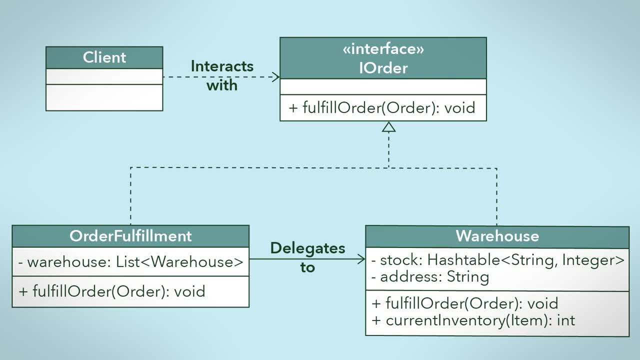 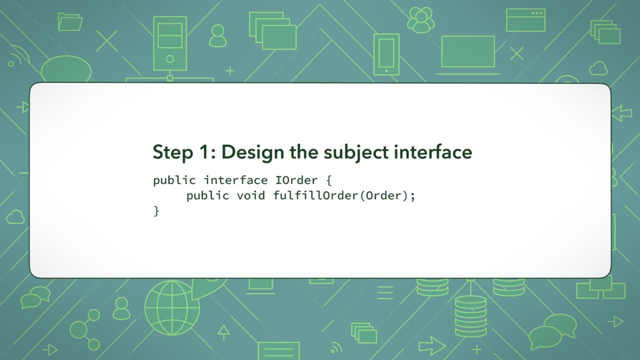 pattern. the client will interact with your system by using the interface. Now that you have completed the design for your Order Fulfillment system, the next step is to implement it. Step 1. Design the subject interface. Create the interface that client. 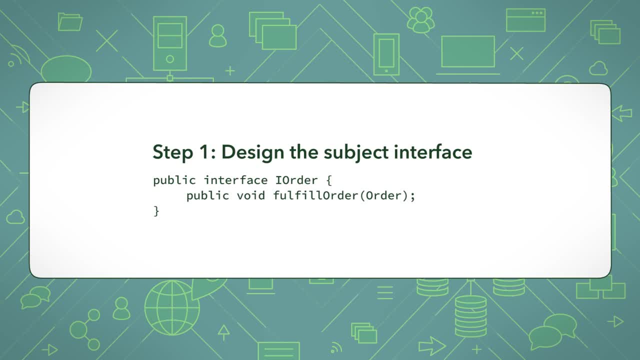 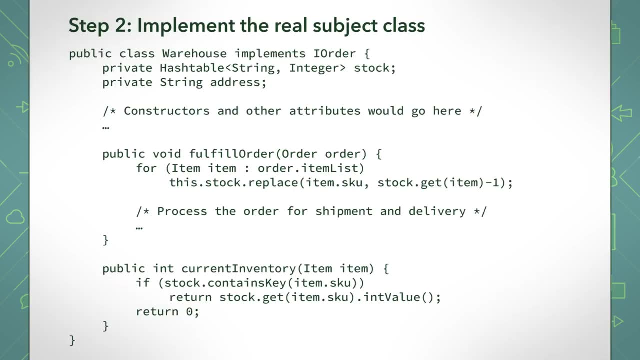 software will use to interact with your system. This interface will be implemented by the Order Fulfillment and Warehouse classes. Step 2. Implement the real subject class. The Warehouse class knows how to process an Order Fulfillment and it knows how to report the current. 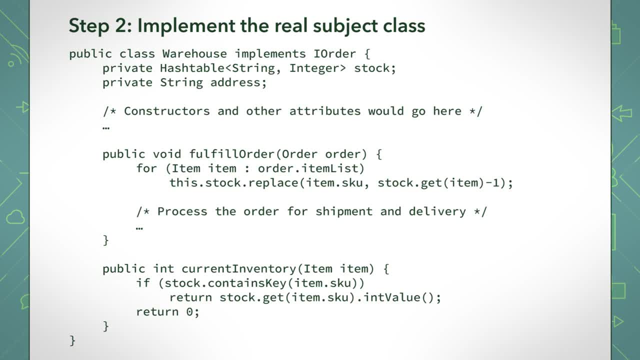 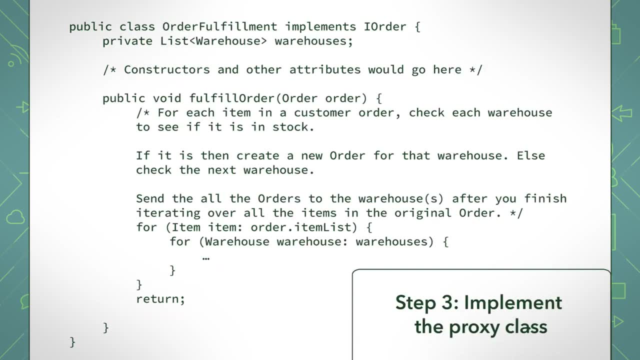 stock of items. Notice that it doesn't need to check if it has enough stock to fulfill an order, because an order should only be sent to a warehouse if it can be fulfilled. Step 3. Implement the proxy class. The Order Fulfillment class does all the work of checking. 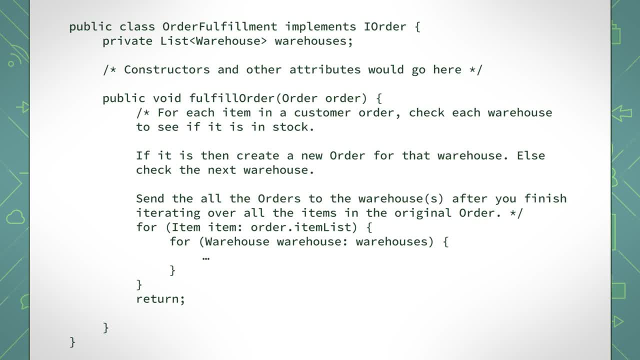 the warehouse inventory and ensuring that an order can be successfully completed. before sending the request to the warehouse, It will ask each warehouse about whether it has enough stock of a particular item. If the warehouse has enough inventory, the item gets added to a new Order object that will be sent to the warehouse. 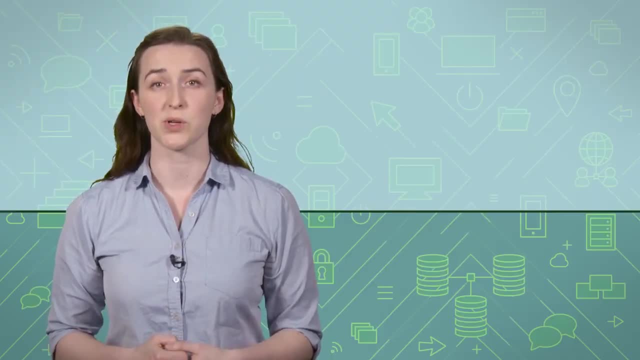 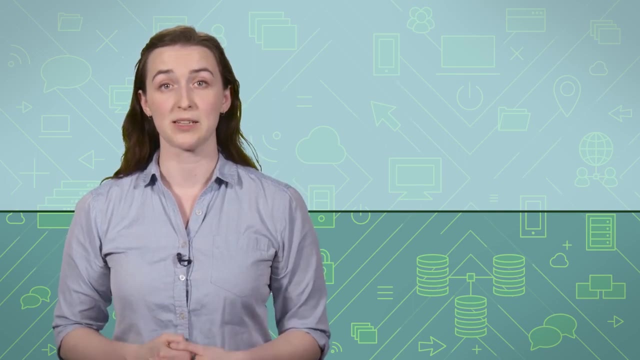 The proxy class ensures that an order can be fulfilled before sending the request to your warehouses. This protects your warehouse system from receiving orders it cannot fulfill. The Order Fulfillment class also lets you separate order validation from the Order Fulfillment by separating them into two pieces. This will improve the overall rate of processing an. order because the warehouse doesn't have to worry about the validation process. Each individual warehouse also doesn't need to worry about how to reroute an order if the warehouse can't fulfill the order. The Order Fulfillment class can be improved with other functionalities, such as prioritizing.